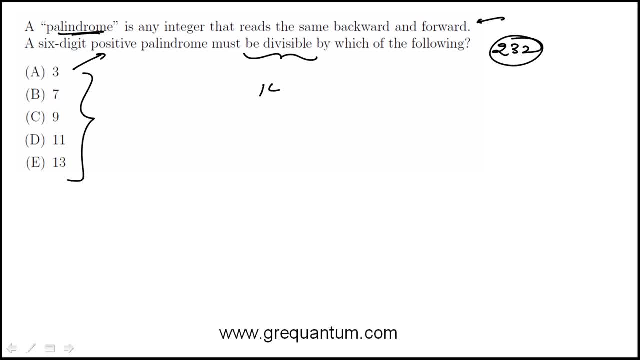 which of the following. So you want to pick up a different example, something like, say, 145541.. It reads the same in both directions. I'm deliberately choosing something different from that, because I know most students are going to do that and you'll see multiple. 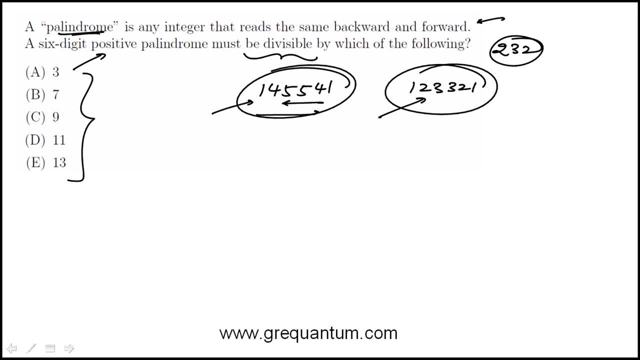 of these numbers will work. Now, if you look at this, I can add up the digits: This is 10,, just this part, and that's another 10.. So some of the digits is 20, and this number will not be divisible by 3, because 20 is not divisible by 3.. Same thing with 9.. The rule: 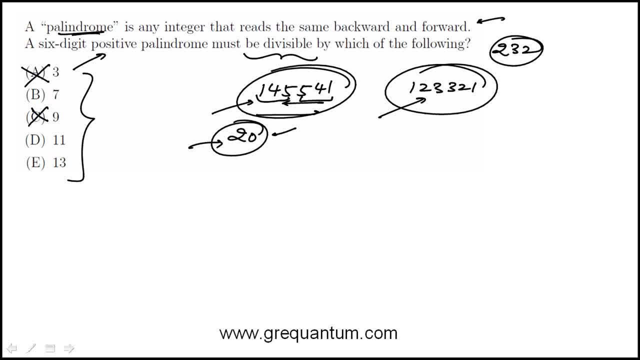 is the same. The sum of the digits is divisible by 9, then the number is also, And for the remaining 3, we'll just use the calculator. If you divide this by 7, it's not divisible by 7.. If you do it by 11, you'll find that. 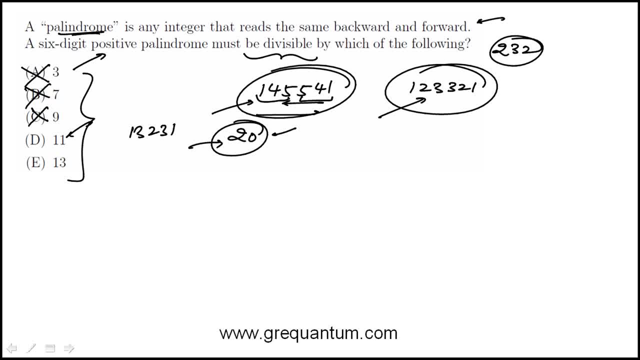 the result is divisible. So we know that this is one possible answer. And then for 13, if we divide it by 13,, you'll find it's not. So we have our answer immediately. But there is a general concept behind this problem that relates to place value, and you might see. 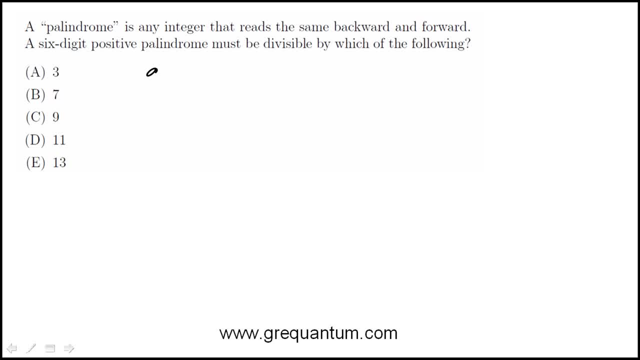 it in a different problem 1, And I want to review that. It's not terribly useful for this particular problem, but it will be useful. So now, in terms of place value, this just means A. this would be 10B, and 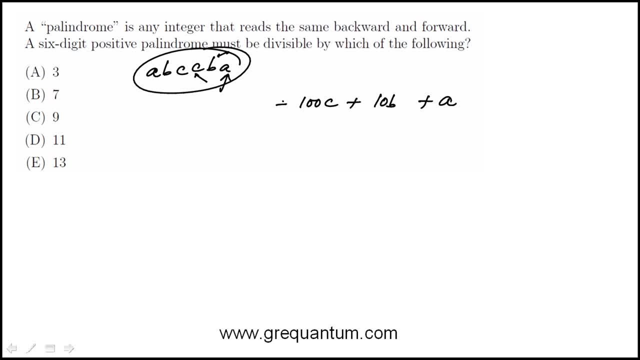 then I have 100C- I'm going from the back- And then plus 1,000C, then 10,000B, and then I have 5 zeros. Actually, yeah, no, this is 6. So I have 100,000A. So this is our number Now. 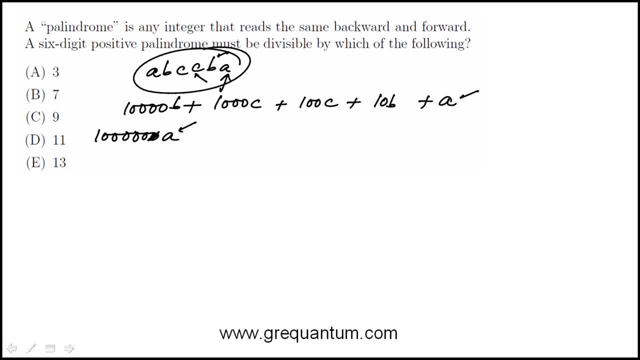 if I were to add these up, meaning combine the A terms, so this would be A and then I would have 10,010B, these two terms and then plus 1,100C. So I want to see what number.